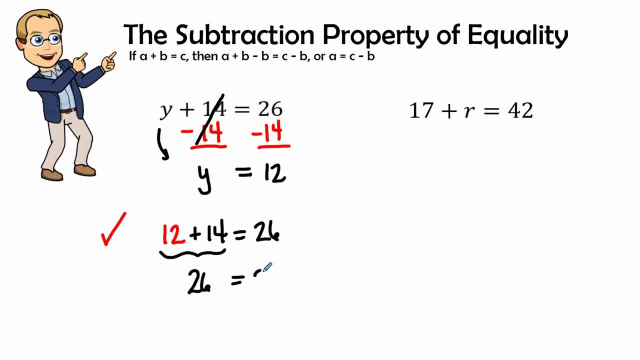 So we see that 26 is equal to 26,. therefore, the answer is correct and it checks out. In our next problem we see 17 plus r equals 42. Now we don't see a sign in front of this 17,. 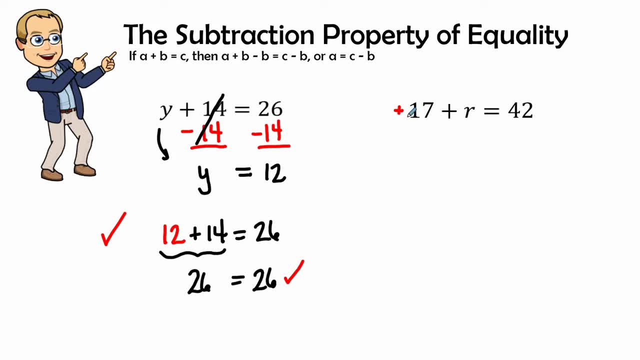 so every time we see- I don't see a sign, I have to assume that it's going to be positive. If it was negative, that negative sign would be there. If it was negative, that negative sign would be there. So what is the inverse of positive 17? It's a negative 17.. And through the subtraction, 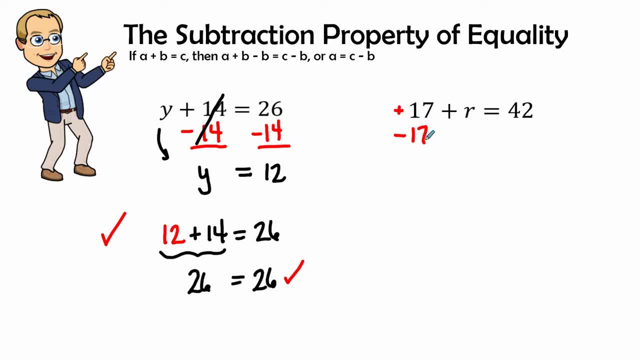 property of equality. what I do on the left side of the equation, I'm also going to do on the right side of the equation, So I'm going to subtract 17 on both sides. Now this is inverse of each other, and when we have a number that- and it's inverse- it always equals zero. So we will have r by itself. 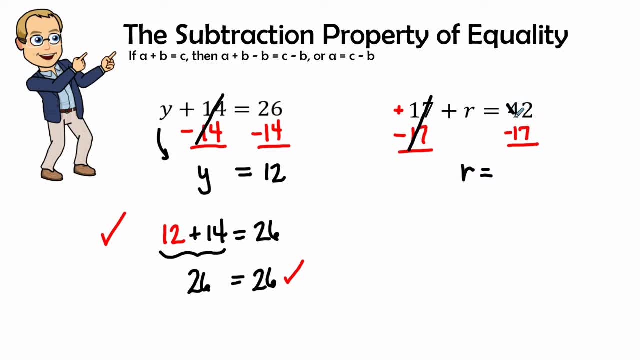 and then we'll have 42 minus 17.. So we can see that we'll borrow 10.. Now we have 12 minus 7 is 5, and 3 minus 1 is 2.. So we see that r is equal to 25.. Let's go ahead and check our work, So we 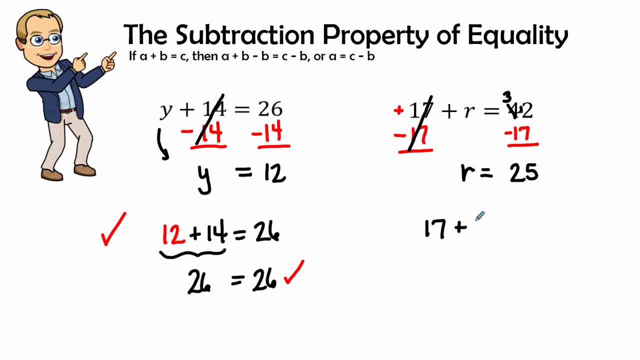 have 17, plus that variable replaced by the r would be 25.. We'll put that together, So we would have 15 plus 5.. So we get it is equal to 20.. Then we have 12 and 3 plus 5. So we get 13 plus 12.. And now we are at 10 plus 4.. So we can see that. 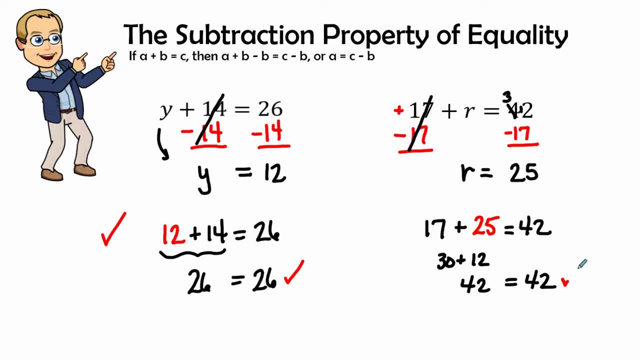 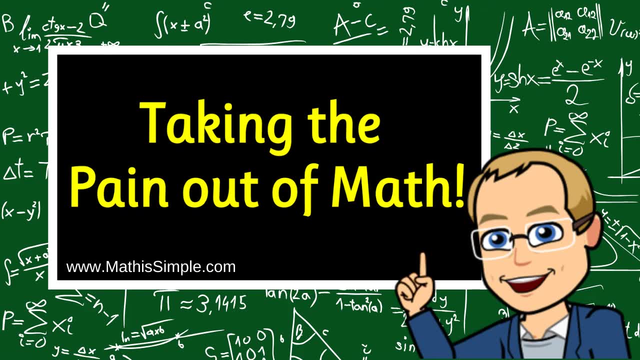 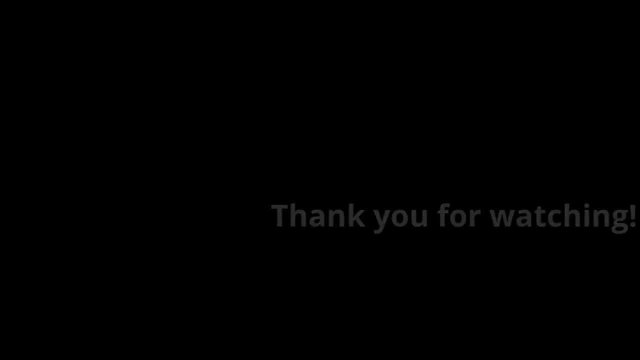 r is equal to 42.. Well, 10 and 20 is 30.. 7 plus 5 is 12.. Therefore, 42 is equal to 42. And we know that our answer is correct. Thank you.